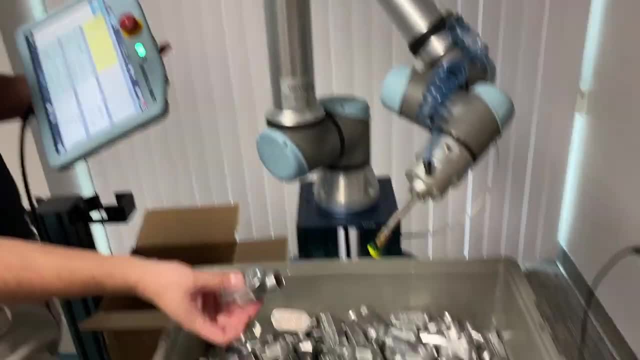 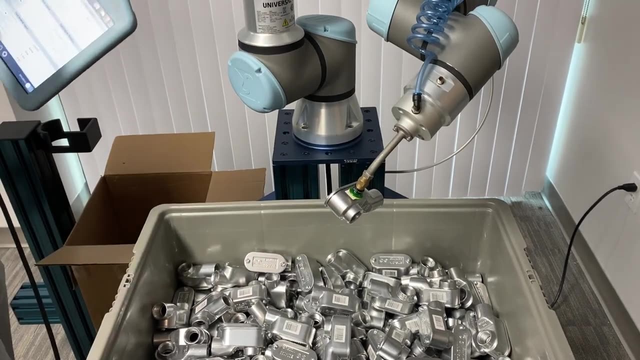 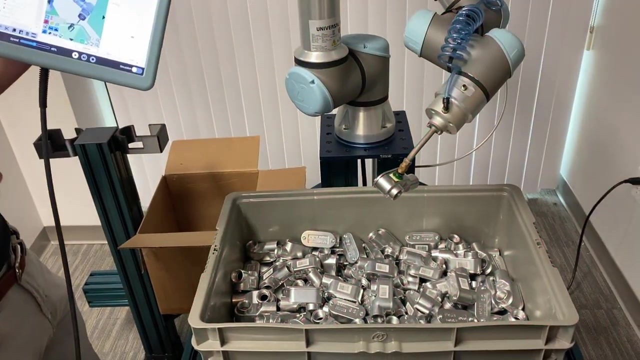 We're going to turn the suction on and we're going to attach the part here in the middle of this barcode, OK, and then we come back here and, like the instructions, say we hit scan. So you're going to see the lights flash when we hit scan. OK, and it's looking for that part and it found it Here. it. 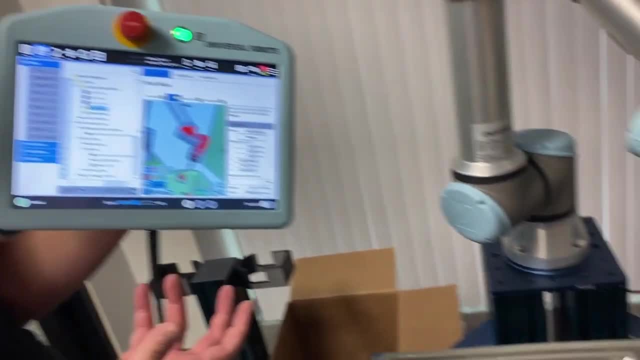 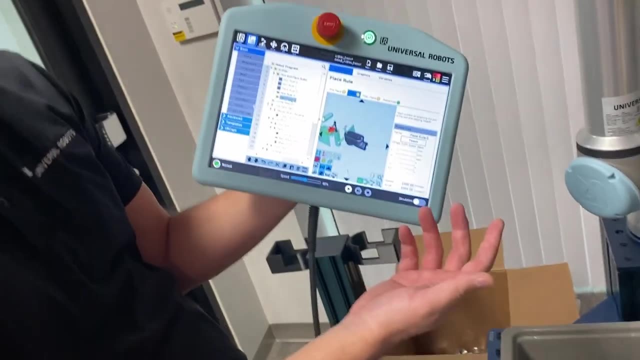 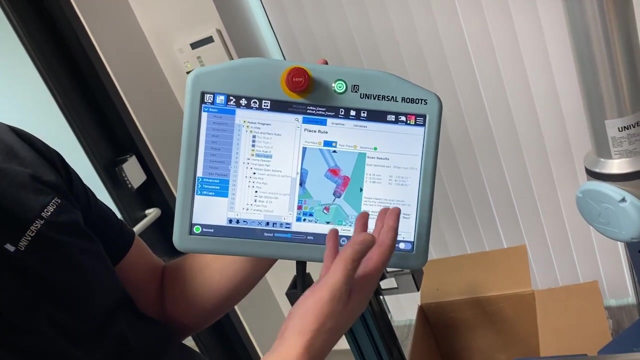 is, And we hit, done. So now we've just trained it to only pick parts here in the middle of this barcode. OK, so the next question is: how do we want to place it? Well, again, the first step is the same: Hit that teach button, hit scan, see the lights flash, finds the part. But now we want to. 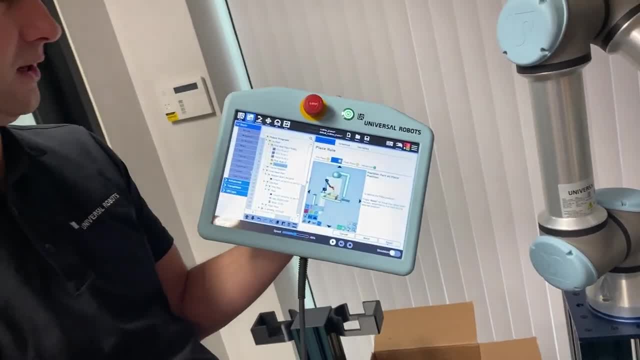 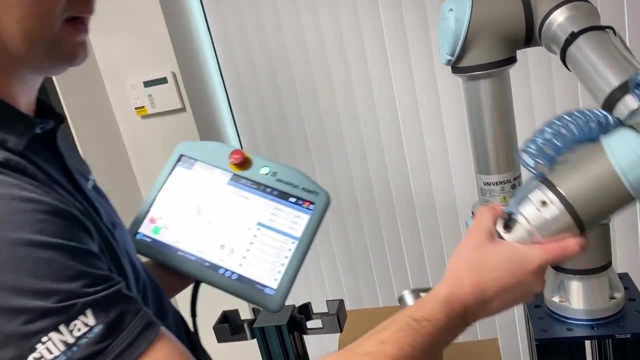 show it where in the world we want to place it: into a chuck, into a fixture, Whatever the case may be. So it tells us to place the part how we want to place it. So in this case, why don't we just place it in my hand, right here, OK, and you'll notice the flat side is facing me. 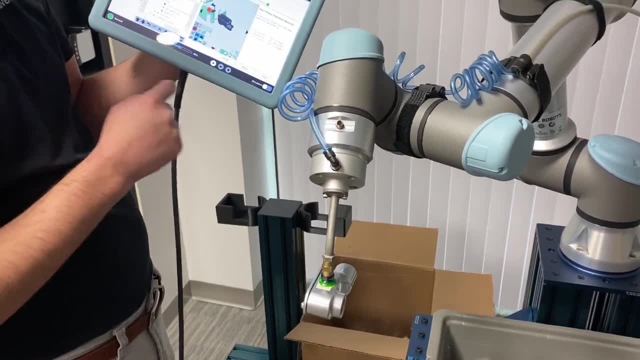 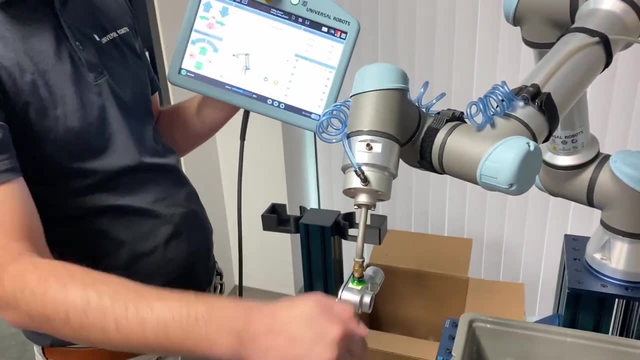 and you know, the two holes, the two threaded holes are facing that way. And then it asks us: what about preplace? How do you want to go into this hand or this chuck? And we want to. we want to come from above, So we want to place it from here. 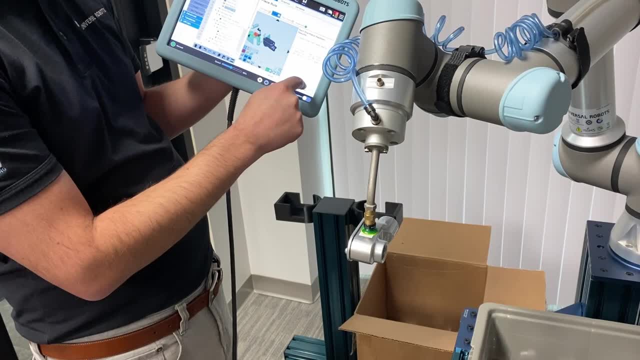 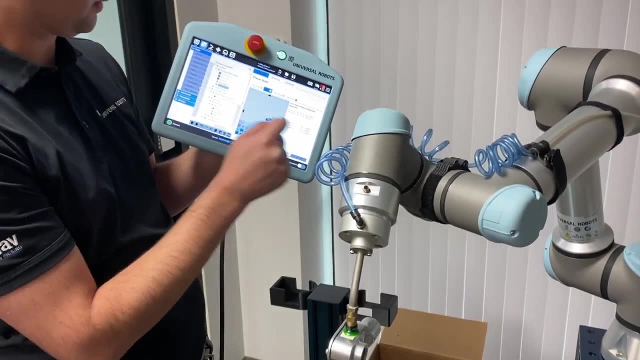 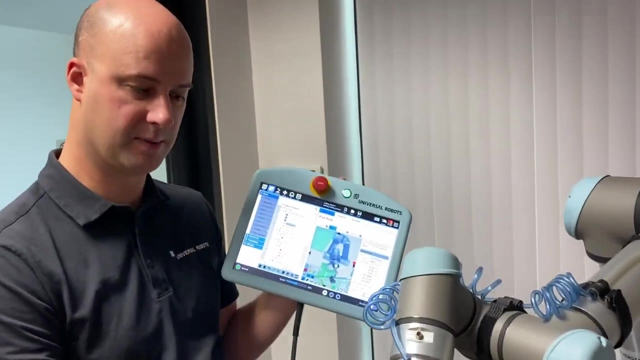 Straight down and we want to go straight back up again. So we want to next set how we're going to go up. Let's say we'll go up two inches and then we'll hit done. And the next thing is you can have any combination of pick rules and place rules, Maybe when you pick the barcode side you want. 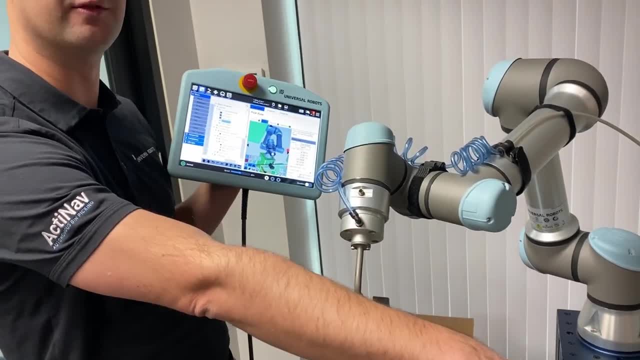 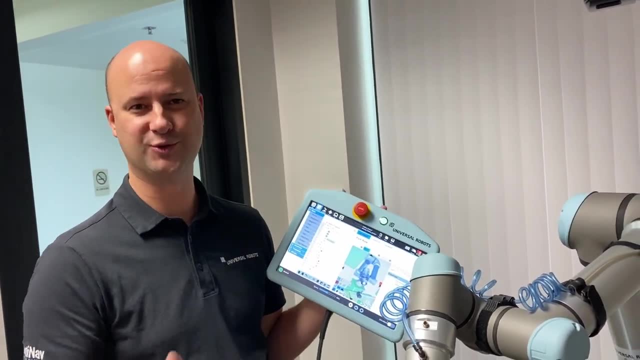 to place it into here, And when you pick the other side, you want to place it over here. So you can have any combination of. you know, pick rules and place rules, So you just link them together for this purpose. We'll just do the simple. 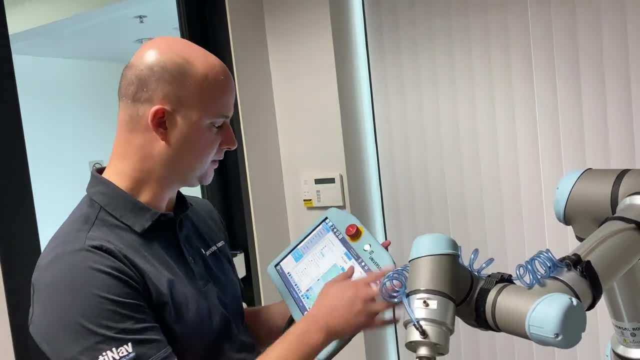 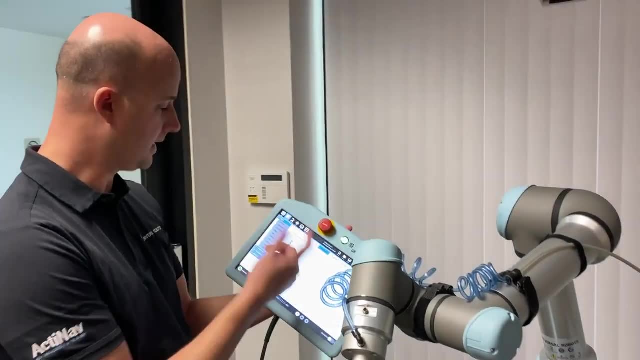 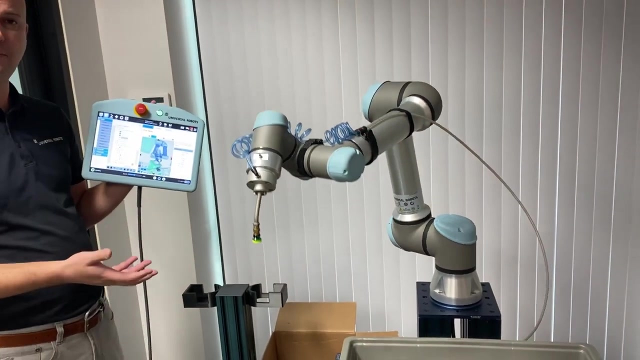 It's dead simplest, which is one pick rule and one place rule. OK, we'll turn the suction off. Good catch, Thank you, And that's it. Yeah, we'll hit play. So the robot's going to go back to home, It's going to scan, It's going to look for parts, that's only looking for. 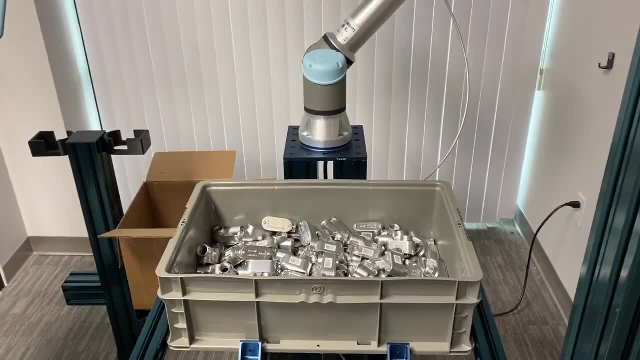 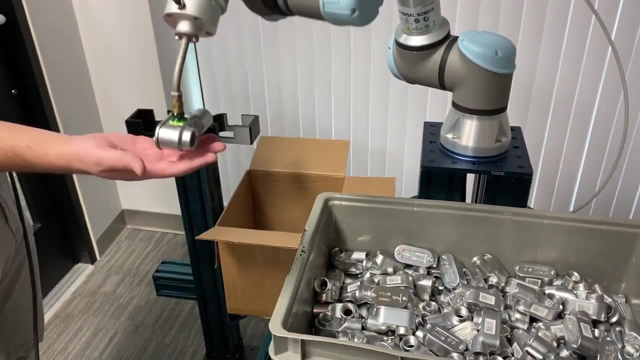 parts with the barcode side facing up, because we only, you know, we only taught it that one. It's going to figure out how to move and it's going to place that part right here in my hand, Again, with the flat side facing me and the two threaded holes facing, facing that way. 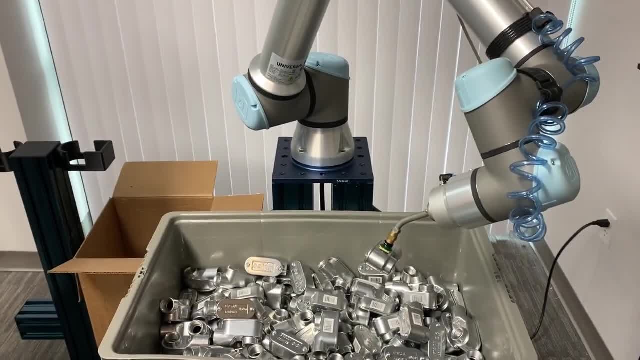 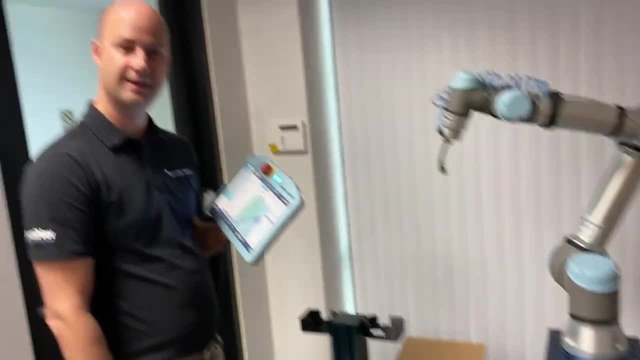 Same configure every time. Yeah, exactly, And so that's how easy it is to train a new. a new pick rule and a new place rule. That's cool, So you can see if you know, part changeover is extremely easy. 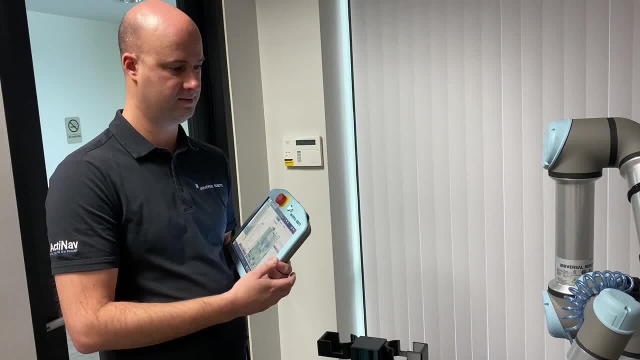 You know you have a new part and loaded CAD model of the new part, You show it. you know three or four different ways where you want to pick it. You show it how you want to place it and you show it how you want to place it And you show it how you want to place it. 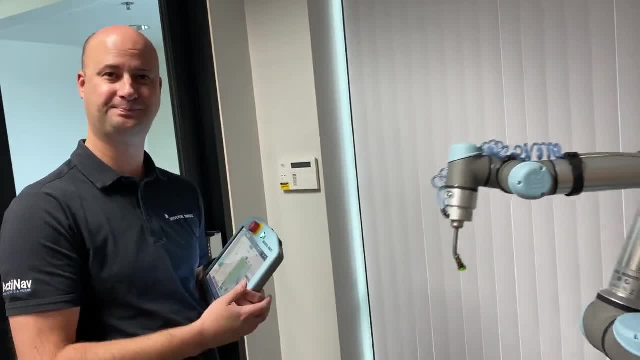 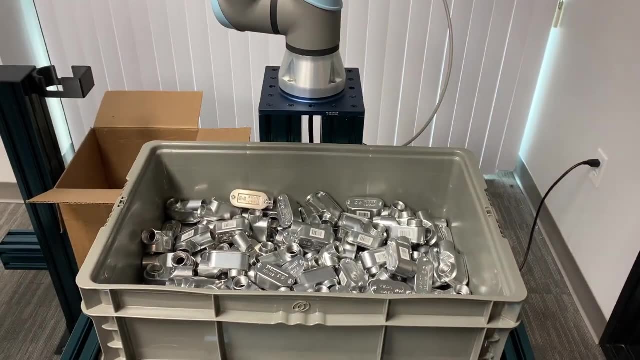 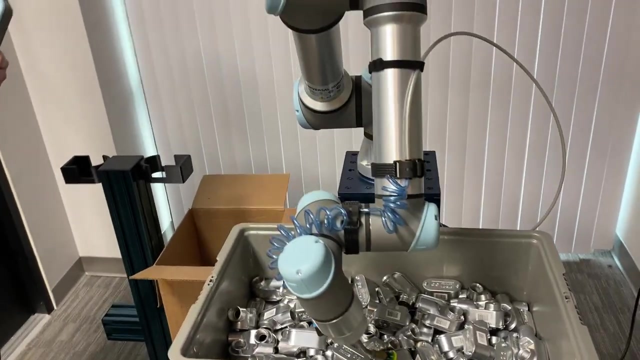 And you hit play and it's going to. it's going to go figure out how to do that. Okay, And one, one last point on those flashing lights. That's a laser scanning this area And you had said before it's it keeps track of the first time it scans and then 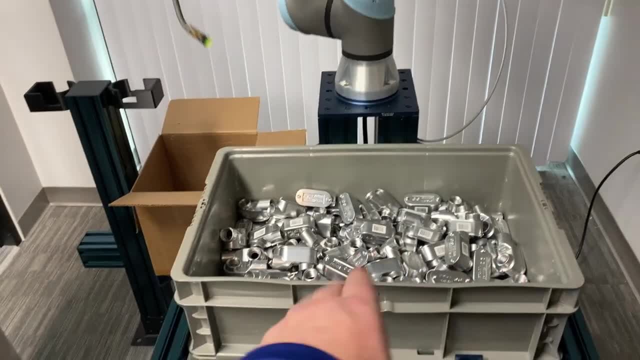 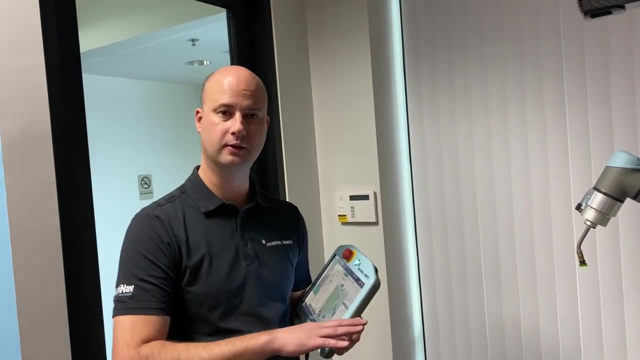 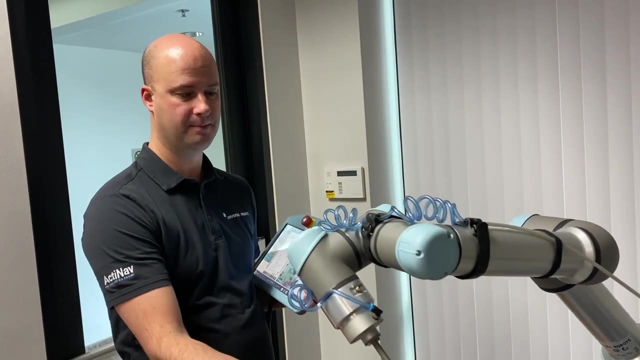 it notices any changes thereafter unless, like you heard happen, there maybe several parts move and then it does rescan like it just did. So, yeah, what it does is it actually looks, you know, looks into the future. you could say So it does scan every single time, But actually 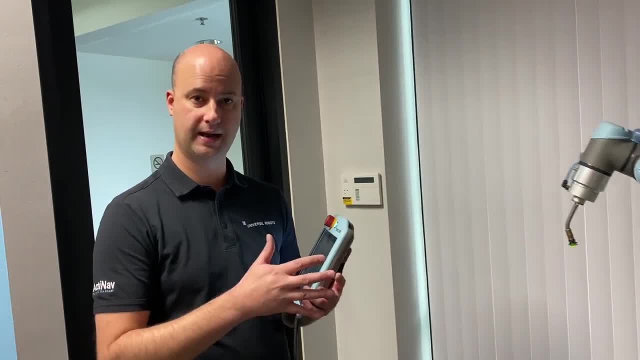 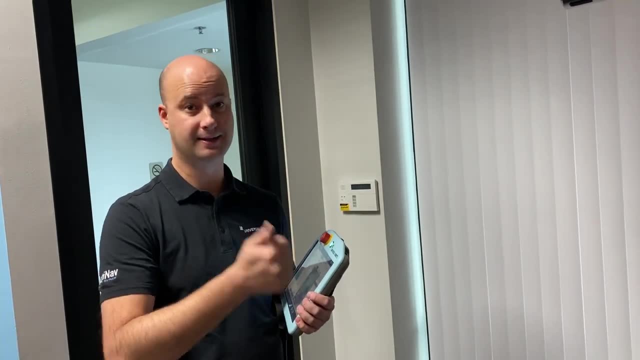 as the system gets gets up and running, it's creating a cache of future picks and paths. So when it scans, sometimes it's just checking: hey, is the? is the part that I've already planned the path to? Is it still there? And if it is still there, it just simply goes and executes. 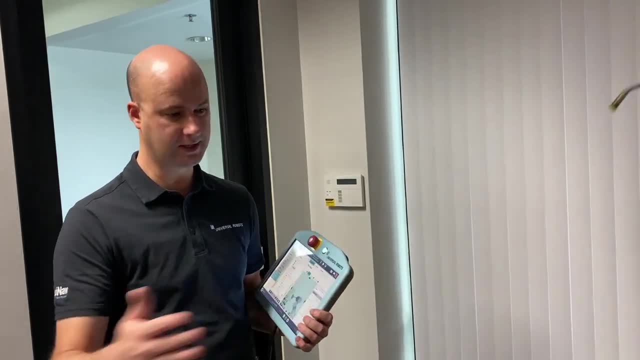 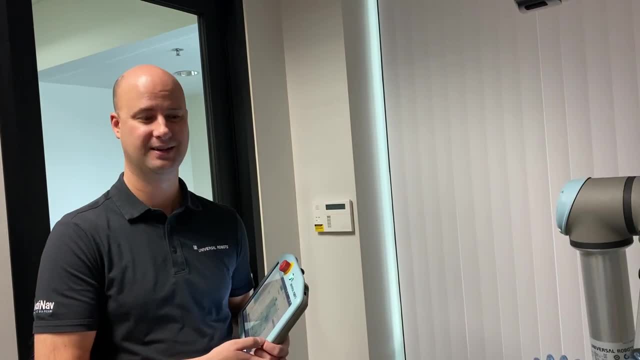 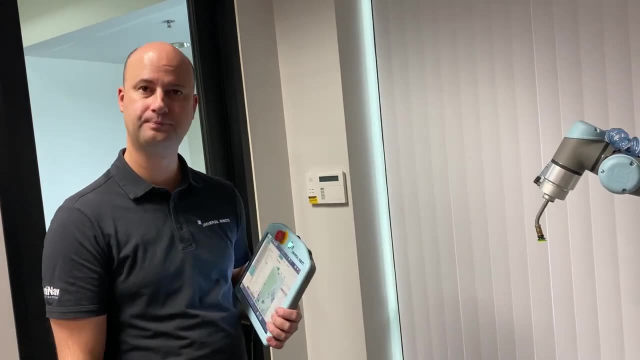 When it scans it says, hey, actually that part is not in the same place that I think it should be, And then it'll clear that cache and start over. Okay, And then we figure the next five steps. and then we figure the next five ones, Yeah.